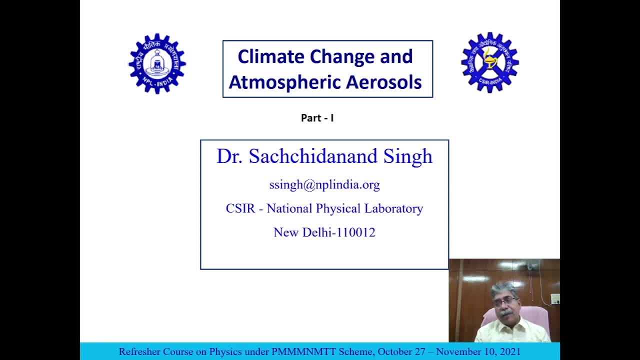 constitutes mainly the lecturers and teachers from different universities and colleges. So it may be a bit difficult for me, as most of our interactions is limited to either the students or the hardcore research group. but interacting with the people who are actively doing teaching and then also involved in research may be a difficult task. but 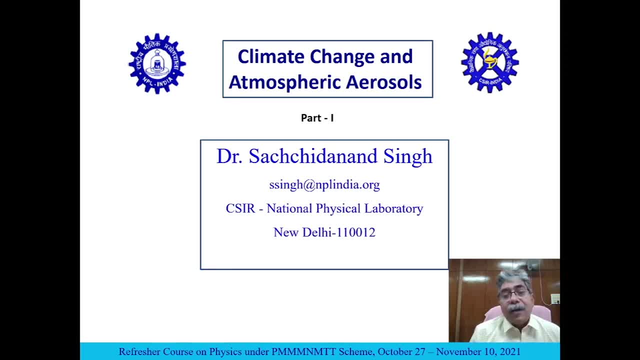 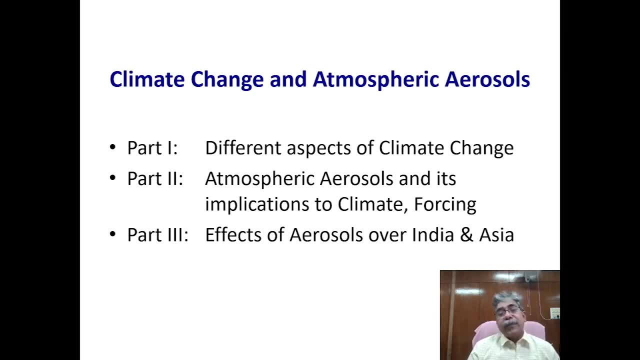 then I would still like to do some justice to you. This talk actually will consist of three parts. In the first part, we'll deal with the different aspects of climate change in general, and then, in second part, we'll discuss the atmospheric aerosols which some of you may 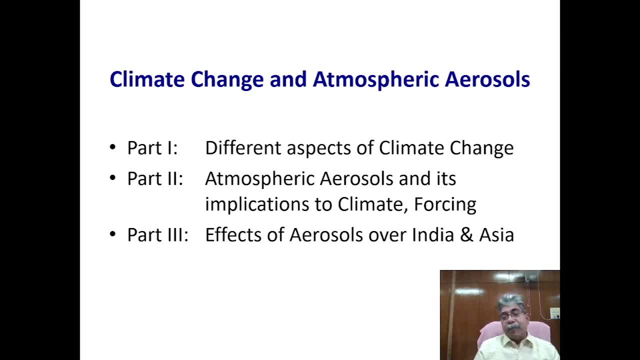 not be aware of in such details which we'll be discussing here. and then it's an implication on climate, say climate forcing, aerosol, radiative forcing, etc. Then the last part, the third one, will be where we'll discuss the effects of these atmospheric aerosols over India, particularly from the radiation perspective and a bit to over. 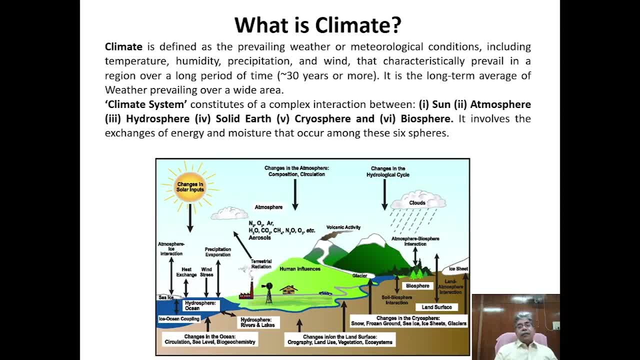 Asia. So now to start with the climate change, the first thing that comes to our mind is: what is climate? and climate is basically defined as the prevailing weather or the average of weather. in general terms, what we can say, that climate is what we expect and the weather is what we get. the day-to-day events. day-to-day events. 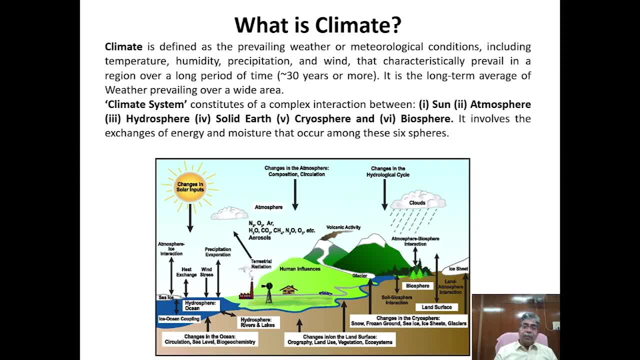 day-to-day changes in temperature, humidity, pressure, cloudiness, etc. It is part of weather, but when we see it on a very long time period and see the average characteristics, then it is what is called the climate. This average is normally taken for a period of at least 30 years, or more than that. So basically the climate, which is the 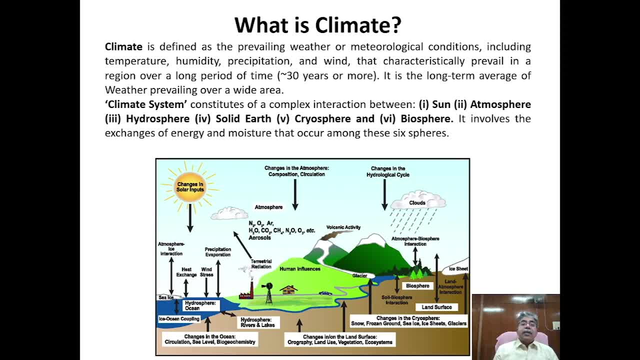 weather, and it includes the changes in the temperature, humidity, precipitation, winds, etc. over a very long period of time and over a very wider area also. Now, this climate system, it takes different, you know, spheres which have interactions between themselves, and these interactions are very complex, which starts from the Sun itself and then the 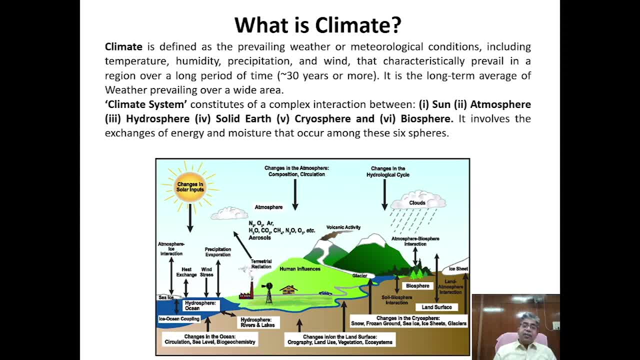 interaction takes place from atmosphere, hydrosphere, then of course the solid earth, cryosphere, and then the biosphere. So it basically involves the exchange of energy, moisture, air, parcel, etc. between these different spheres of climate system and which, in the interaction with each other. 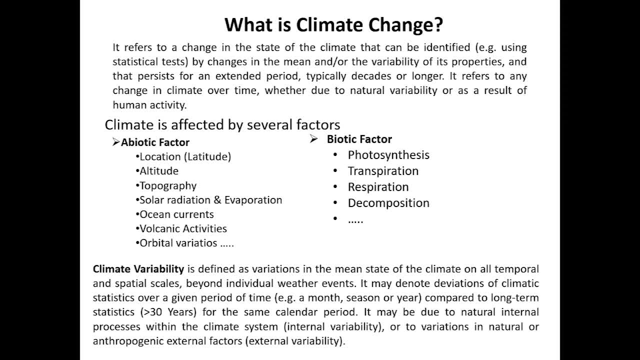 give rise to what is called the climate over a long period of time. Now the changes that we refer into. this climate is basically the state of the climate, which can be identified through statistical tests or by changes which can be observed in the mean variability of different properties. and then 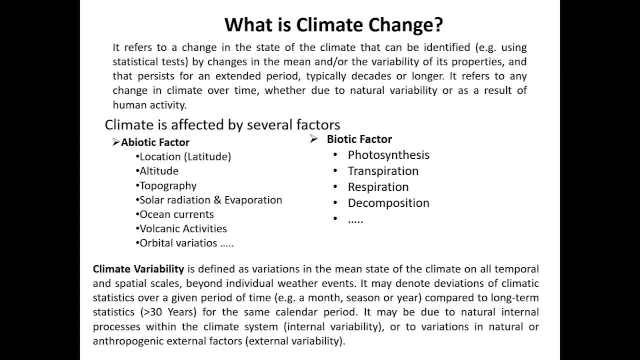 over an extended period of time, So typically over a decade or maybe longer, then such changes actually refer to the climate change. So these changes may be because of the natural variability or it may be a result of human activity. So depending upon that, it is basically divided. 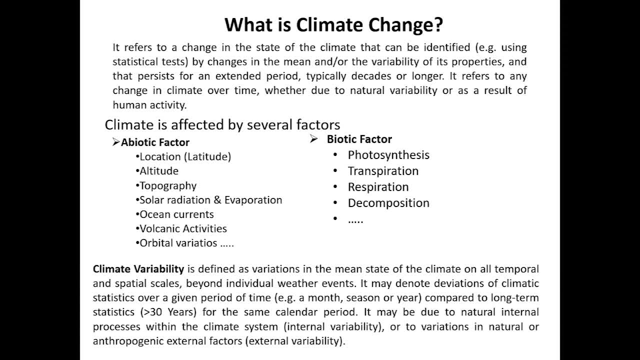 into two kinds of factors which can affect the climate. One is say abiotic factors, which are its latitude, longitude, topography, solar radiation, then volcanic activities or ocean currents, etc. On the other hand, the biotic factors may be: 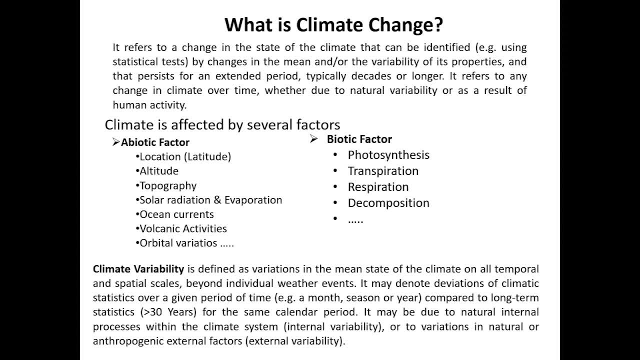 the photosynthesis, transpiration, respiration, decomposition, even the natural decay process, like that. They all contribute towards the climate change over a long period of time. But then this climate change starts with a fluctuation in the climate, or which is called 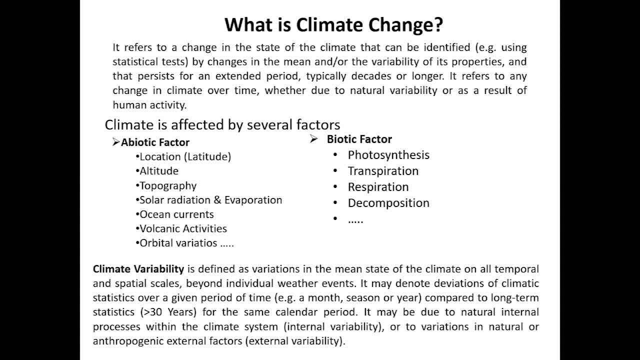 the climate variability and which is actually defined as a variation in the mean state of climate on different temporal scales. So it can be anything between a day or for a longer period of over a year, But then it is beyond the individual weather events. So anything it can denote will have. 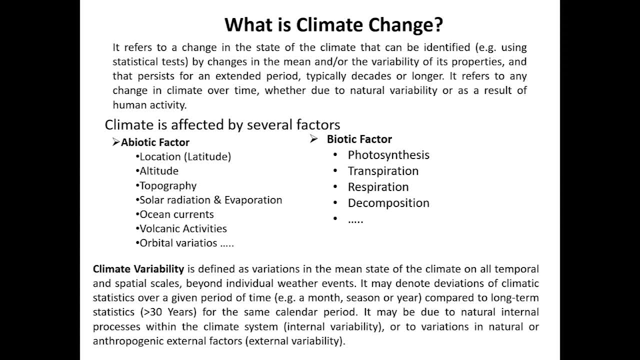 a statistical averaged time period for more than 30 years. So even if we are talking about a change in climatic variability on a monthly basis, the average time period will be more than 30 years, or on a seasonal basis, then it has to be an average of more than 30 years. 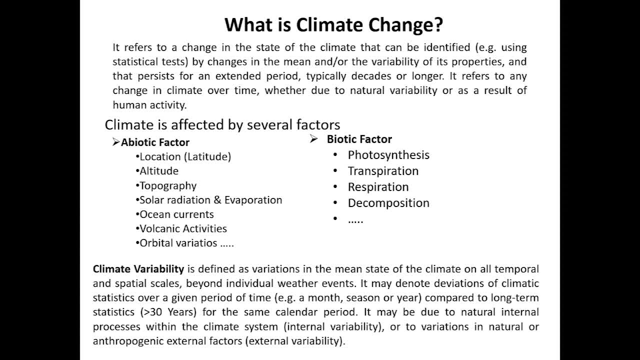 behavior of climate variability, and then these. these variability may occur because of the internal factors of the entire climate system, which is then called the internal variability, or due to the various natural or anthropogenically external factors. the natural external factors may be volcanic eruption or something like that, and then anthropogenic activities are. 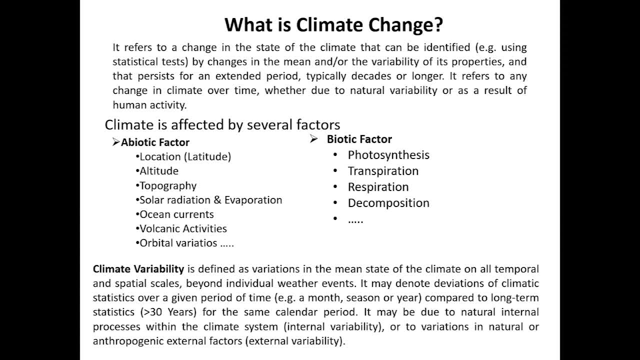 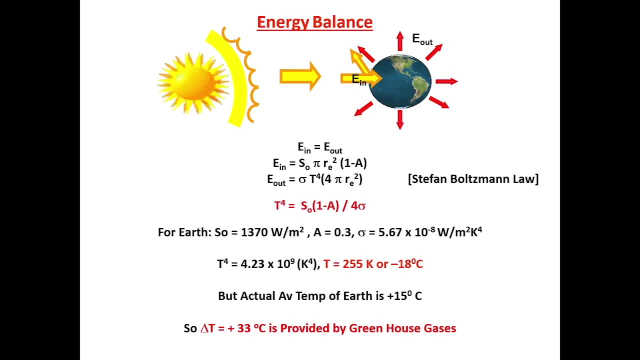 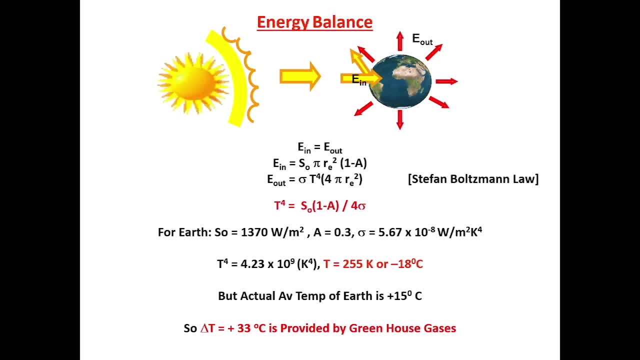 the the the result of the energy balance which always exists between the Sun and the earth, in this case, in our case. so, whenever the net amount of, as we know, the net amount of energy which is incoming to the earth, earth and Earth's atmosphere must be equivalent to what is going out of the earth through radiation, 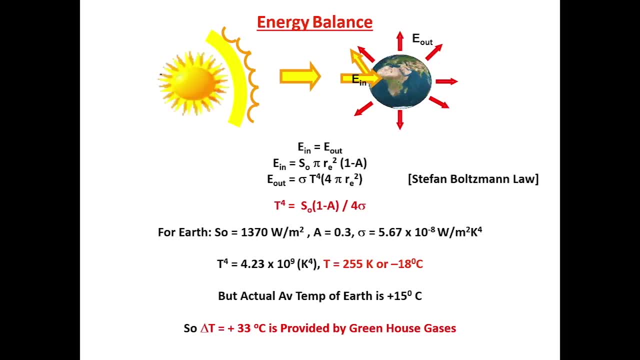 and when we equalize these two energies through mathematical formulations using the Stefan Boltzmann law, then what we find? that the temperature of the earth it should be about 255 Kelvin, which is around minus 18 degree centigrade. so here we have taken the. you know, the, the, the. 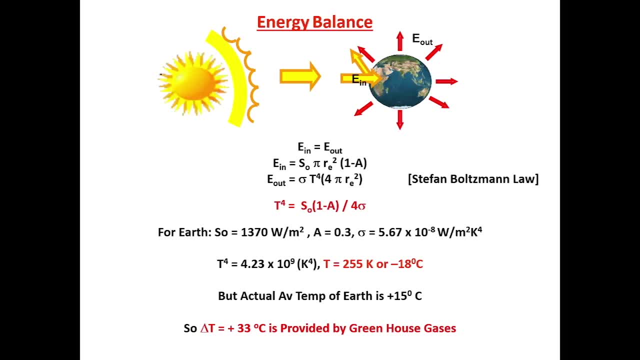 amount of radiation which is, on the average, falling on the Earth's surface is 1370 watt per meter square, and which is true also, and because of that, the average temperature should be minus 18 degree centigrade, which you can also say is the temperature of a perfectly black body, which is at a, which will have the 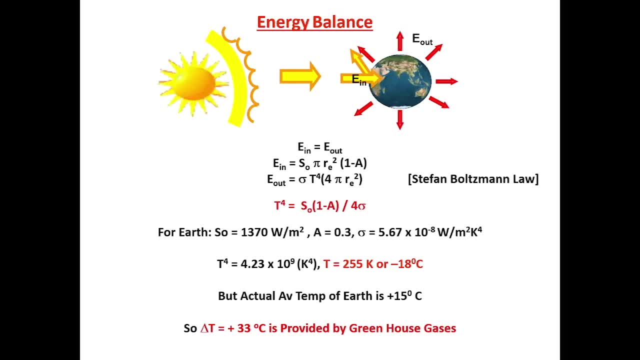 temperature up to 35 Kelvin, but the actual average temperature of Earth is about 15 degree centigrade, and so a net difference of about 33 degree which is observed between the theoretically obtained temperature of the Earth and the average temperature of the Earth if target of the surface east, for example. 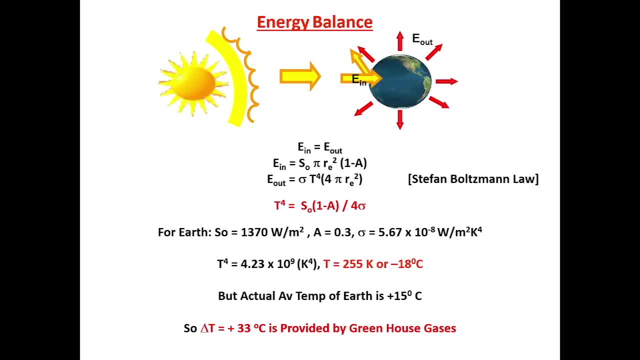 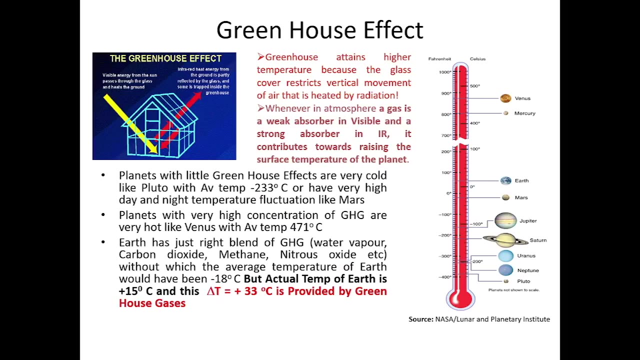 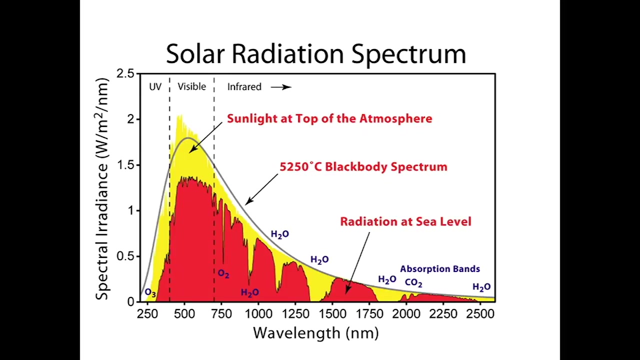 the actual temperature of the earth, and which is 33 degree centigrade, and this difference is actually provided by the greenhouse gas which exists on the Earth's atmosphere, and that is what makes this planet livable, as we have seen in previous slides. so, and this black curve denotes the blackbody. 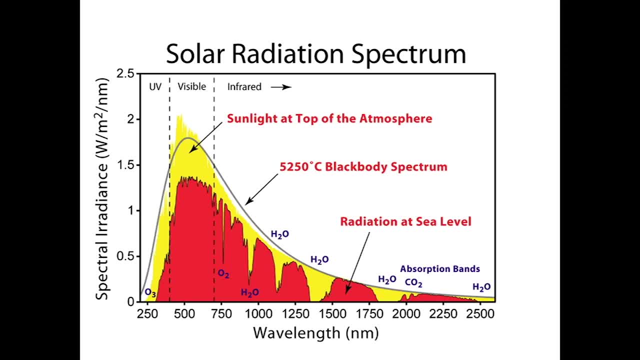 spectrum at 5250 degree centigrade, which is roughly the surface temperature of the Sun, and then the red curve is what the radiation is obtained at the sea surface, over the earth, and you can see that there are various absorption bands. there is a lot of absorption due to different constituents, say for 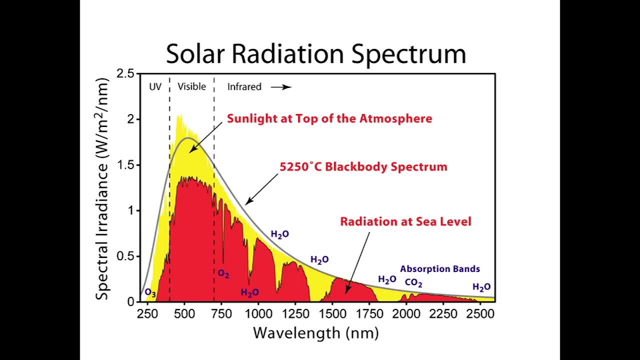 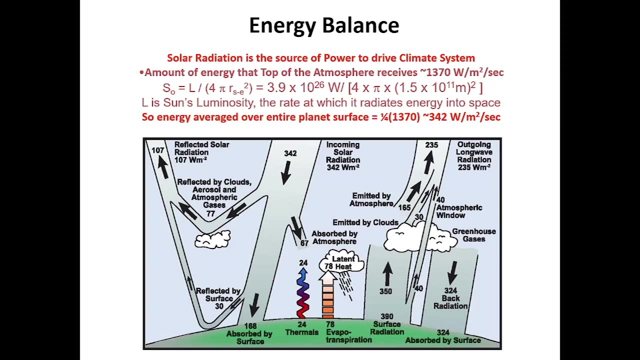 example, ozone, then water vapor, H2O, CO2 and so on, so forth. so these are the basically greenhouse gases which absorb the longwave radiation and which give rise to the greenhouse effect that we have seen earlier. now the important thing is the energy which is falling at. 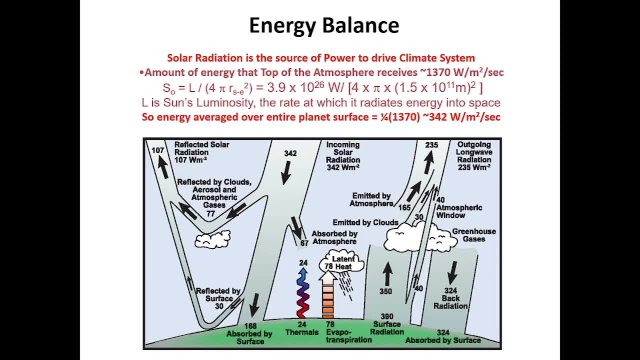 the surface is eventually re-radiated back into the atmosphere, and this balance of energy is always maintained because the energy at the top of the atmosphere is about 1370 watt per meter square per second, and earth, since it is rotating and it is falling over the entire surface area of the earth. so 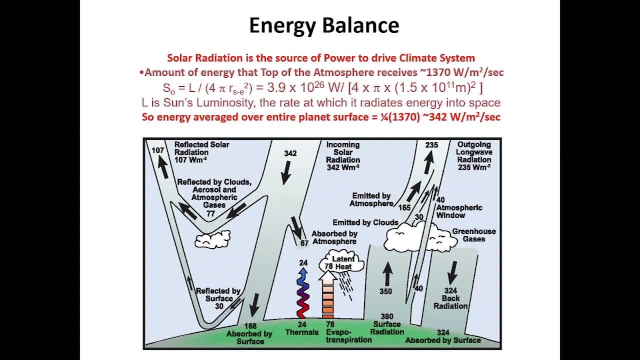 basically the when we make the these calculations. so then it is actually the 342 watt per meter square per second of energy which is being received on an average at the entire surface of the planet earth, and this 342 watt of energy received is actually- again, it is a redistributed back and is given back. 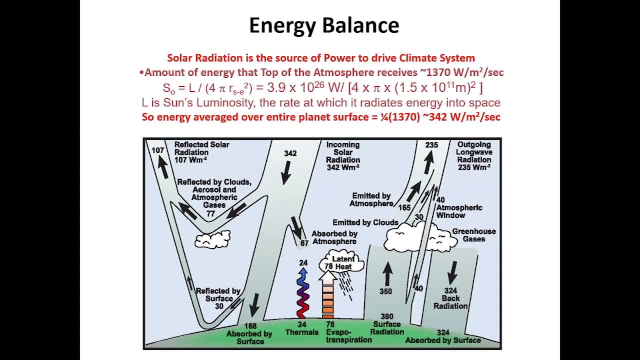 to the atmosphere. so out of this 342, around 107 watt is reflected directly from the surface and clouds and different reflecting mechanism of the surface and atmosphere, and then the about 235 watt is the net outgoing longwave radiation which is re-radiated by the earth due to 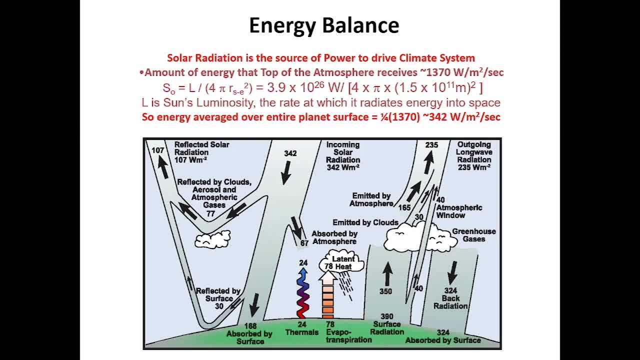 its temperature and due to its temperature of different constituents like clouds and other things. in between, there is a redistribution of the energy which, in the form of latent heat, which is actually emerging from the surface, in the form of water vapor, and so so, eventually, the net effect of this energy, 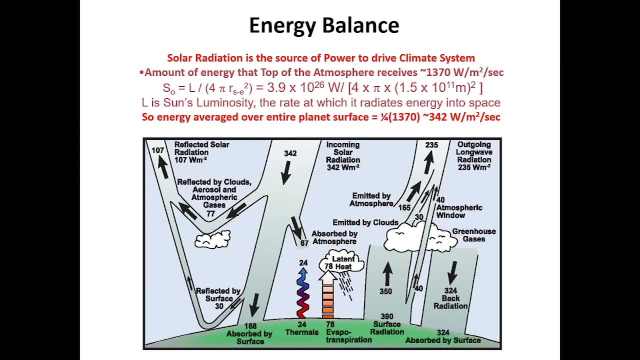 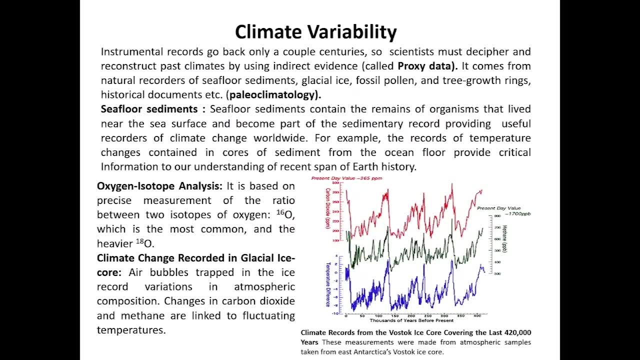 balance is that the whatever amount of radiation which is received is actually given out by the earth and its system. now coming back to the climate variability: climate variability is not a new thing. it has been happening over the ages and we have seen that, although the observations are available only over a 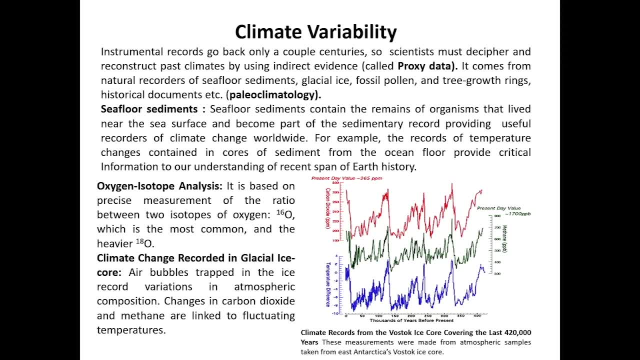 few last couple of centuries. but there are various proxy data, proxy data which are the data which can be inferred from the past- climatic records or past through various processes. so from those proxy data we have, the scientists have seen that the climate of the earth has kept on varying on a very large scale and it has been 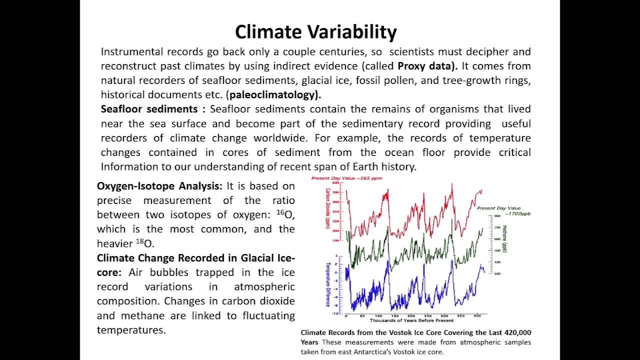 happening from ages. in here particularly, you can see that when they it comes to the natural record, so that we are, which are available by scientists now, and because now we are able to explore more and more through different scientific techniques which are available to us, so even through seafloor. 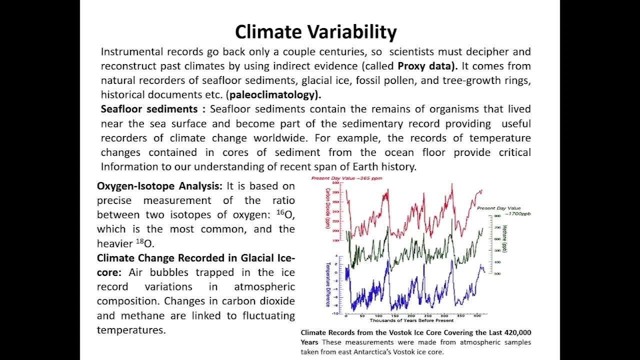 sediments or glacial ice, cold drilling or even studying, by studying the fossils of pollens, the tree rings and so on, so forth, the we can have the knowledge of paleo climatology and the scientists have seen that the climate of the earth is different from the climate of the earth and in the past we have been able to. 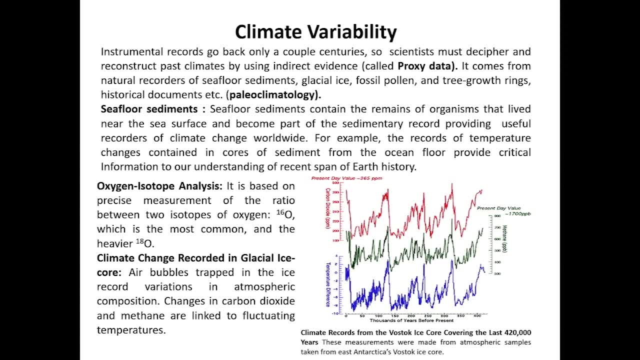 observe almost a textbook and a lot of research. that discovery has shown that, over say last 4 lakh, 20,000 years of climatic record can be obtained through, say, high school drilling, and it has shown that almost the the concentration of major the greenhouse gases like carbon dioxide and methane, they, although have 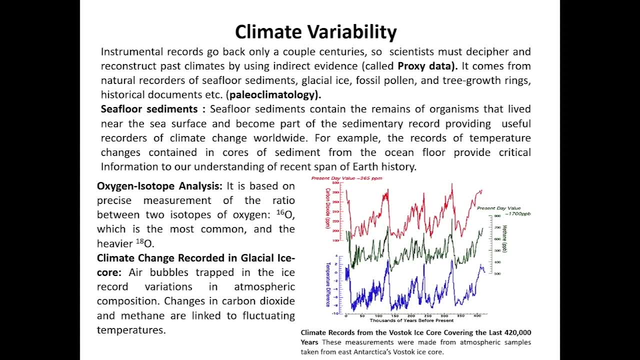 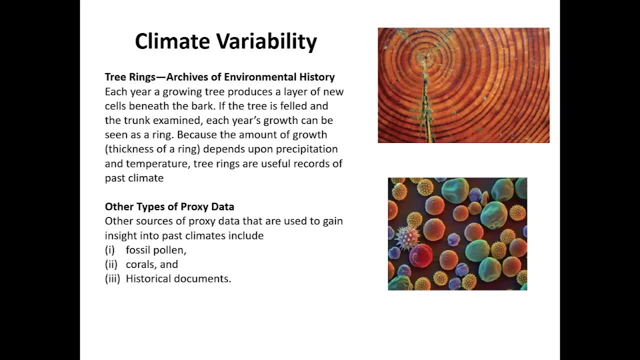 But they remain by and large constant till the start of, say, industrial revolution. And these climatic variability say different methods, as we discussed. one of them was the ice core drilling and the other is the study by studying the tree rings, because, depending upon the availability of moisture, particularly the flood and drought conditions, these various 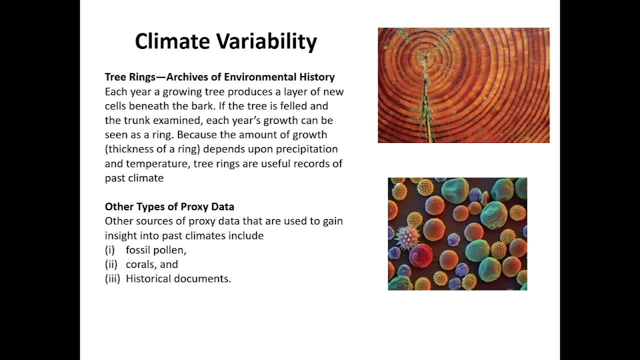 rings on these tree have different widths and by studying those old trees one can study basically the climatic conditions existing at that time. So they are useful records and the past climatic studies are done. We are studying these tree rings. apart from that, there are fossil pollens, corals and 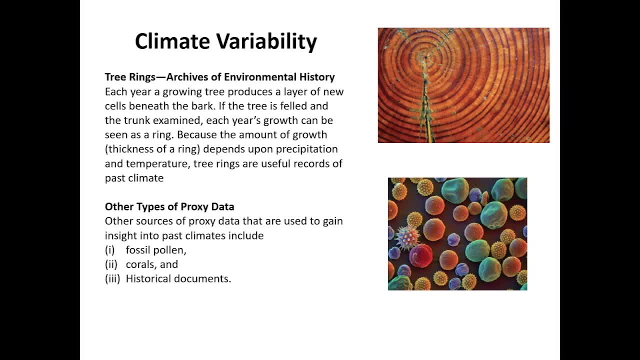 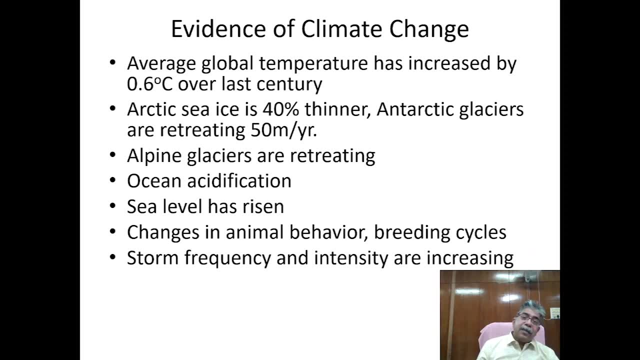 then historical documents through which paleoclimatic changes can be studied. There are several evidences of these paleoclimatic changes, and we have seen that average global temperature over the period of time has increased by about a degree in the past century. They are considered to be the highest temperature in the world. 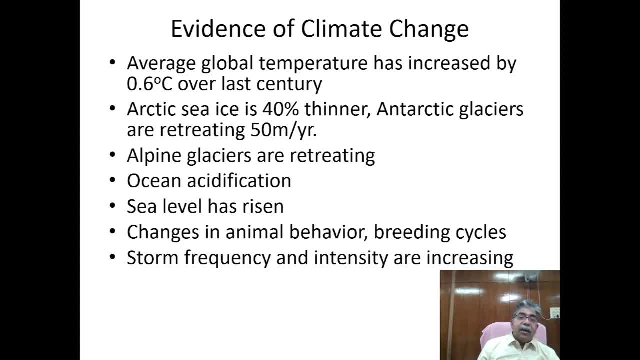 They are considered to be the highest temperature in the world. So the climatic ice is melting and the glaciers are deteriorating at the rate of, say, 50 meters per year or so. Then there are oceans, which are becoming more acidic. Sea level has risen. 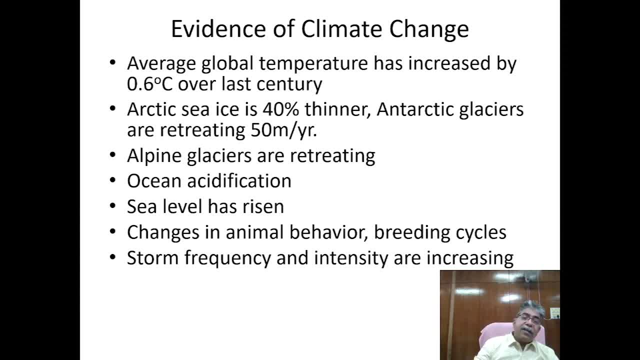 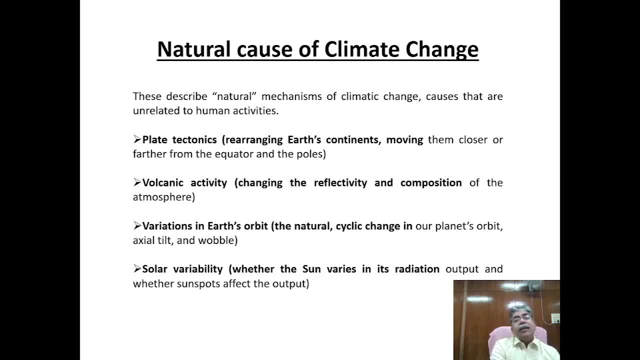 So there are variety of things which provide evidence nowadays that actually the climate change is happening and it is true, The various natural causes of climatic change Which are, as we have discussed, that some of these natural changes where people have no control, and these natural climatic changes are due to many factors. 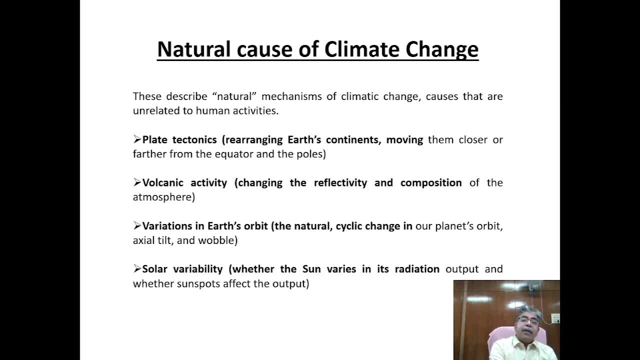 Say one of them is plate tectonics movement, Then the volcanic activities, Then there are variations in Earth's orbit which takes place on a longer time, Then even the solar variability, or the sun of spot number variability, which are supposed to be giving rise to this climate change. 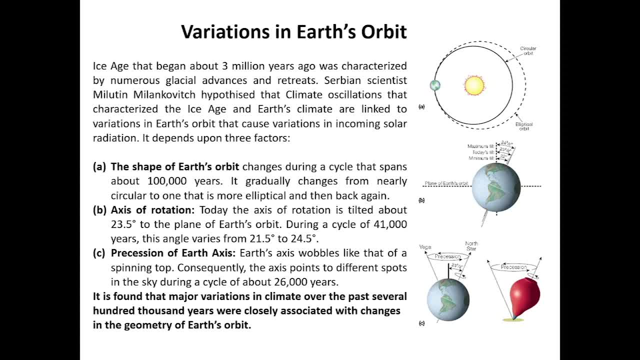 So some of these we will discuss here and which are more important, like the variation in the Earth's orbit. So here you can also talk about the radiations, and there are some BILLIONS of radiations on the earth, From about 3 million years and so on, so forth. 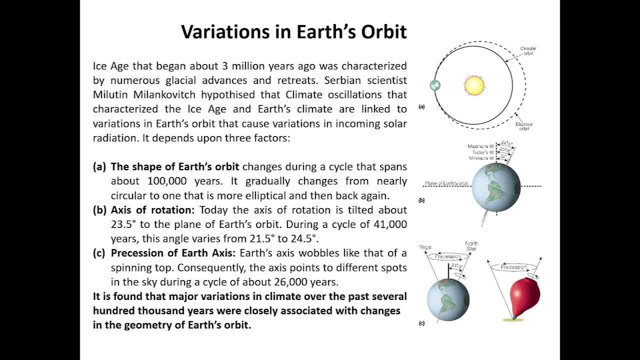 It is believed that some of them can be because of the variation in the earth's orbit And the Serbian scientist Milankovic, He first time proposed the idea that these ice is related to the ice on the earth, And he is a scientist. He has done a lot. 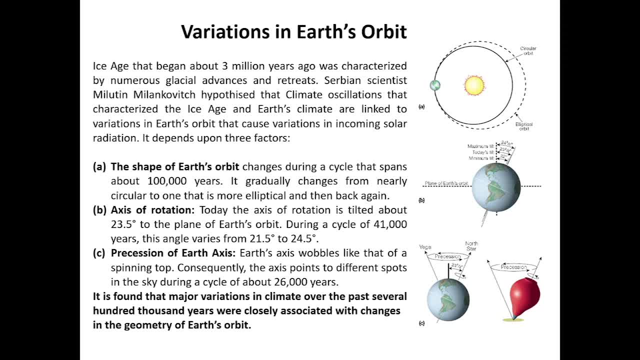 He has done a lot of activities. climatic changes which takes place over earth because of the shift in earth's orbit and which causes the variation in the incoming solar radiation. So this basically depends upon three different factors which can be. the one is shape of the earth's orbit, which changes on a very 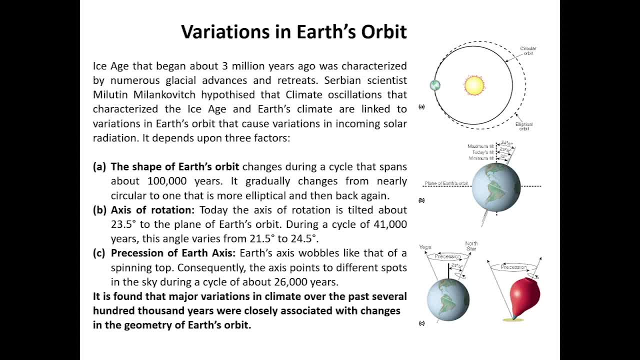 long cycle of, say, about 100,000 years, and gradually, because of this change, the orbital of the earth becomes more elliptical, and then again it goes back and becomes less elliptical, and so over a period of about 100,000 years. Then the another change, which is because of the axis of rotation. 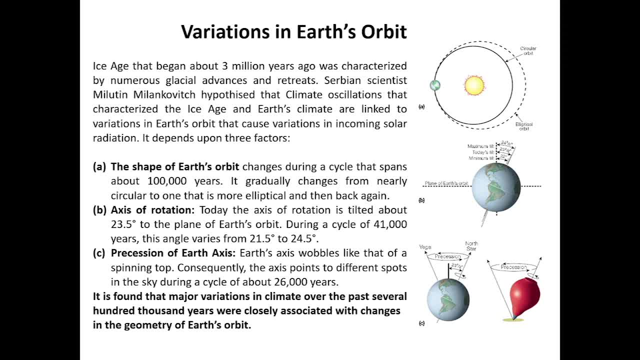 because the earth axis of tilt at which it is rotating also keeps on varying, and it varies in the range of say, 21.5 degree to 24.5 degree. Currently it is about 23.5 degree angle at which this, the axis of rotation, is taking place. but this change in